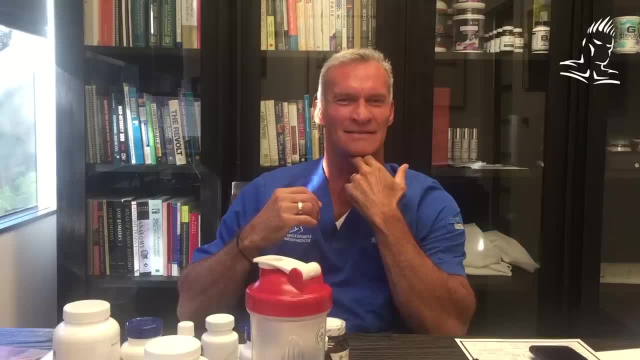 stay in the safest site possible. Thanks in advance, Jonas. That's actually funny, yeah, because I don't know what site he's on, because Boldenone is somewhat similar in structure to Tremblone, right? Oh, really, I don't know. 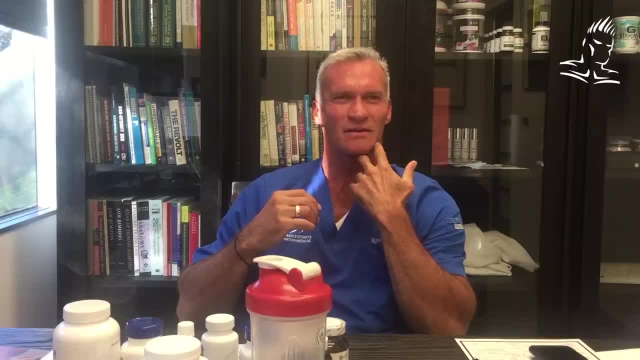 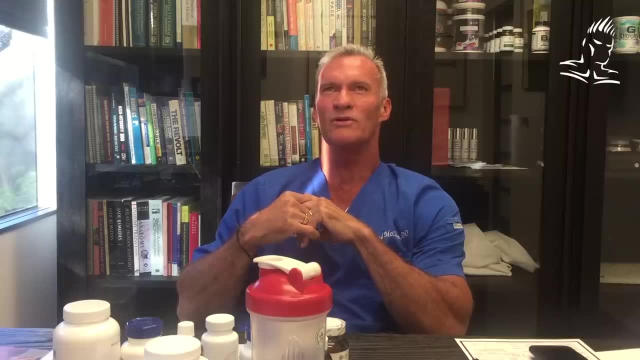 Are they both 19-nor derivatives? I thought one was more. I mean more pre-contest, one more off-season. a little bit. It's been a while. but Boldenone is, Tremblone is the old- I mean again my generation called. 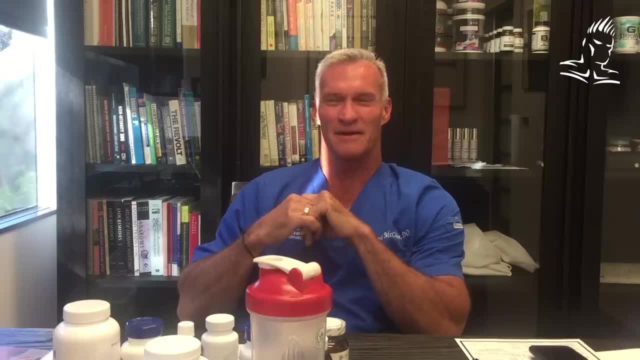 it Parabolin or Phenogen? Yeah, that was the good stuff. Well, it's supposedly all the same stuff and it actually was used on humans before Now. of course, it was contraband in this country and I'm not sure if it's even used. 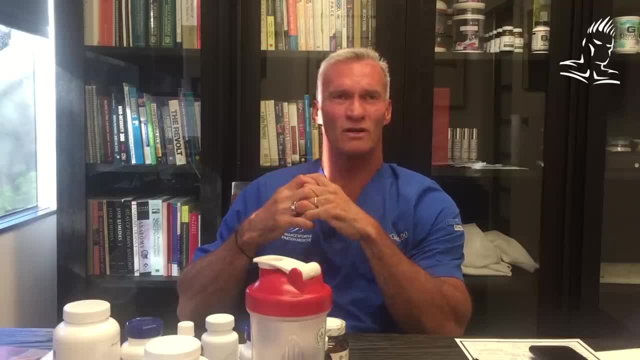 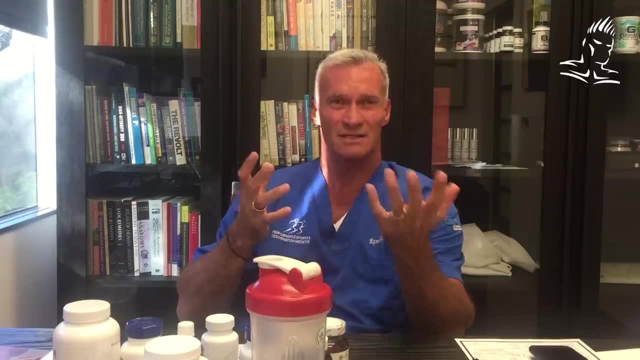 for veterinary use anymore. Ditto for the Boldenone. I think it was also used. it was used to be in a undecanoate form, so it was a long-lasting, you know. I guess it still is. I don't know if they make it any other way but the long-lasting ester, but the Boldenone. 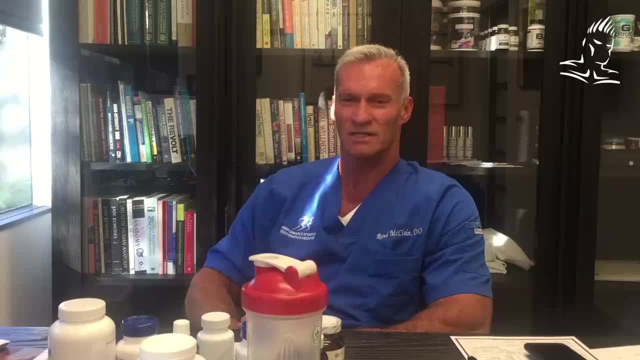 or Ecopoise, is an old drug that actually, from my understanding you know some of that- is actually naturally produced in the human body by the action of 5-alpha reductase on another androgen, But Boldenone. Boldenone is a variant of Dianabol and Dianabol has more of the androgenic side effects and 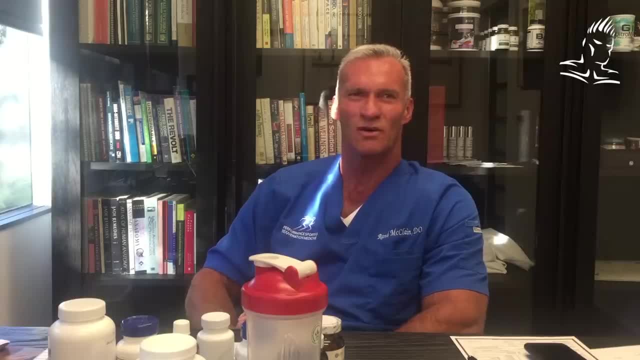 ability to convert into estrogen than Boldenone has. so and of course I think the well, we're not getting too complicated. There are some other issues concerned with any oral anabolic steroid, but also particularly Dianabol with its alkylation. 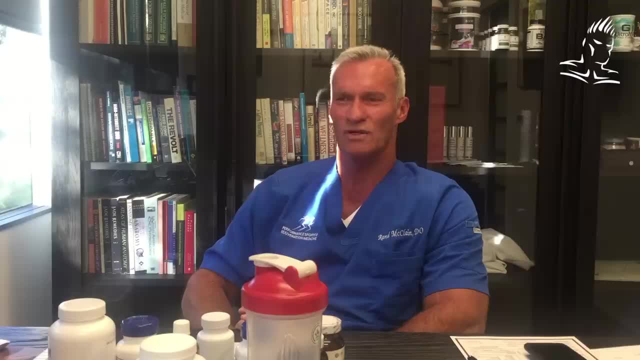 But you know, you certainly don't see that problema anymore and Boldenone is a little bit safer for that. But anyway, Boldenone is a very good anabolic steroid, but it's no longer used for humans, no longer produced for human use. 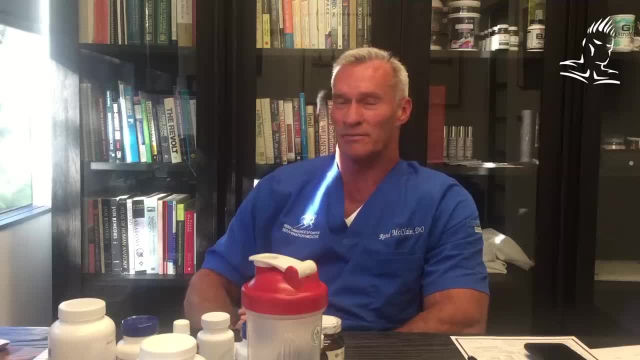 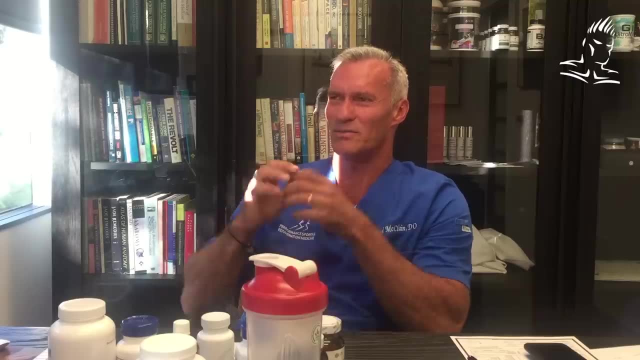 I'm not even sure if it is still produced for veterinary use in this country anyway, but so it's considered a. I don't know where this gentleman hails from. He doesn't say: Anyway, it would be considered a. I think it's considered contraband here. 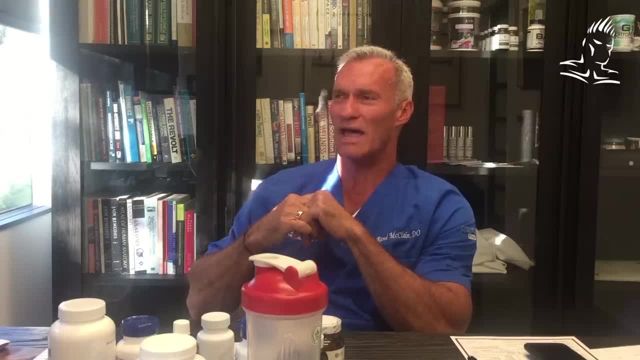 But any rate, it's not absolutely. it would be a fairly safe one. it's got a very long half-life. so if you're talking about dosing, equipoise, um you know, contrary to what you might read, um you know, 200 milligrams would go a long. 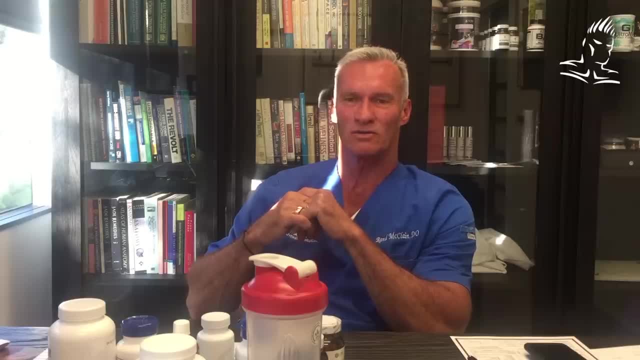 way it's usually in the uh and undecanoate, so it's a very long uh lasting, takes a long time to break down the ester. so, uh, you know, 200 milligrams every two weeks would be plenty, wow, um, yeah, uh, you know. again, i don't know what comes up with the logic otherwise. but uh, there are the protocols, but uh. 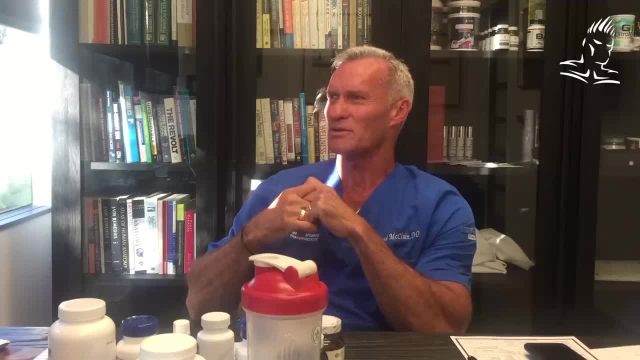 you know trend blown. i think they mentioned trim blown. were we talking about trim alone? yeah, he was asking. he was he didn't want to go that route. he felt it was safer to go with that. well, an interesting choice, because trend alone is a derivative. uh, it's very similar to nangelo. 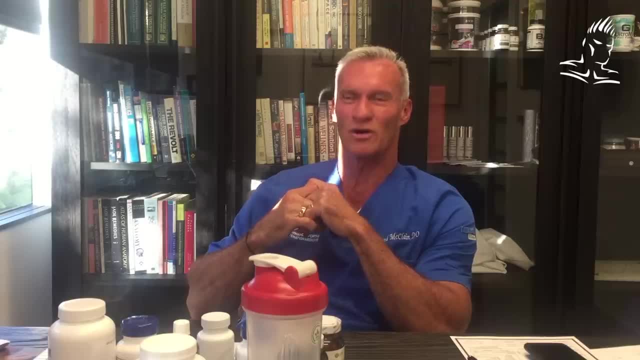 it's a um, uh, you know, we call it 19. nor, and there's a lot of um, a lot of benefits to the that type of steroid also, um, but um, trim balloon, uh, you know, which is, is what used to be called phenoget, and in one form, and parabolin in another form. uh, again used for humans before, but no longer. 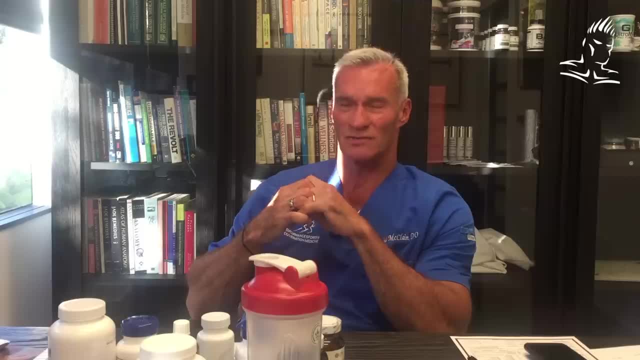 and again i would. it's definitely contraband in this country. i'm not even sure again if it's used for veterinary purposes or not, but um, trend balloon is is very uh, anabolic as well as very androgenic, and it has a very strong affinity for the receptor site. a lot of side effects. 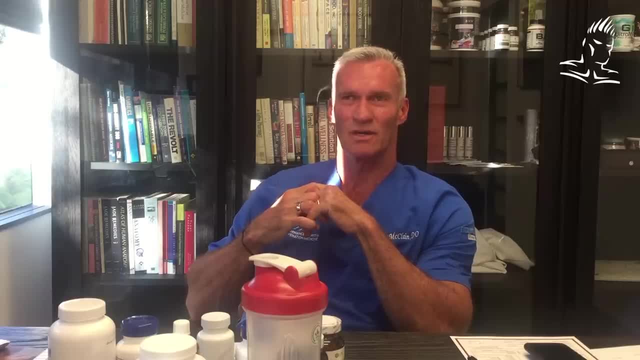 that most people suffer with when they use trim blown, such as profuse sweating at night- a really bad attitude. it can make you pretty aggressive. it's one of those that can you know everyone's different but can have, more likely than not, pretty bad aggressive profile attached, so not one of my favorites to recommend to anybody. 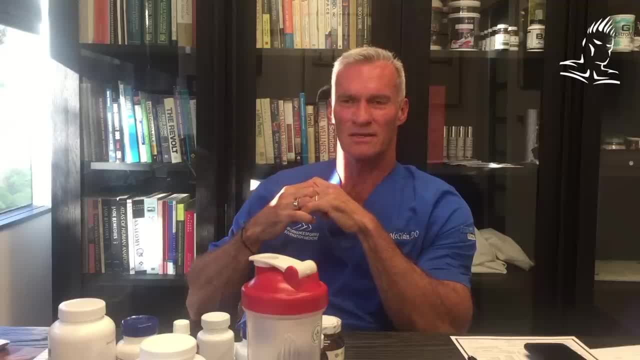 you know, under, theoretically or otherwise. because of that, the um- that said, i mean a lot of body blowers- are very successful with it because it does such a great job prior to a well coming into a show, similarly to the way maybe anavar, followed by winstraw, would really be helpful coming into a. 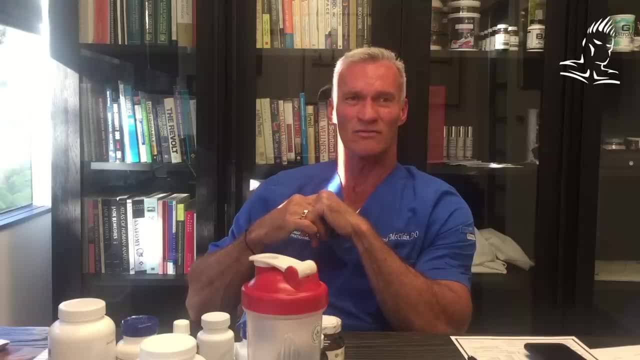 show to help get you lean, get rid of visceral adipose tissue while still acting as an anabolic, or even develop more muscle tissue and also, as they say, dry you out the way winstraw does, which is, you know, is for it's indicated for angioedema amongst its anabolic properties. so a lot of body. 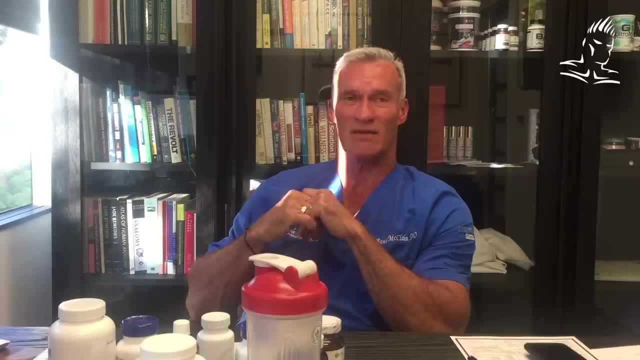 builders, i know, use trend balloon, for example, for 18 weeks out from a show as opposed to going. you know, anavar 18 weeks out and then winstraw six weeks out for that last little bit and getting rid of water. but in terms of you know, if you're just starting out, i don't know why you'd want to go. 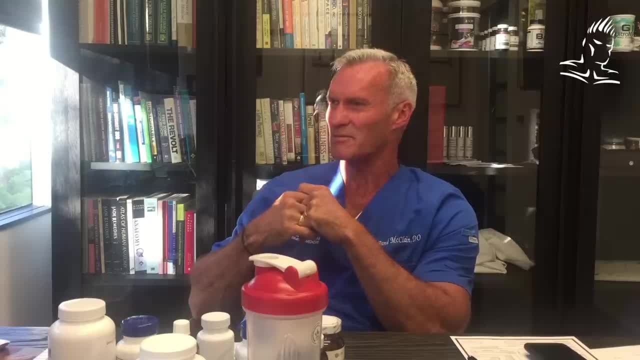 certainly with with something like trim blown, which you're saying. i don't. i don't remember reading it, but yeah, he doesn't really want to do it, he'd rather go with the, the bolden on, based on the way you write. yeah, i mean it's a fairly safe one as far as they go again all these things when they're. 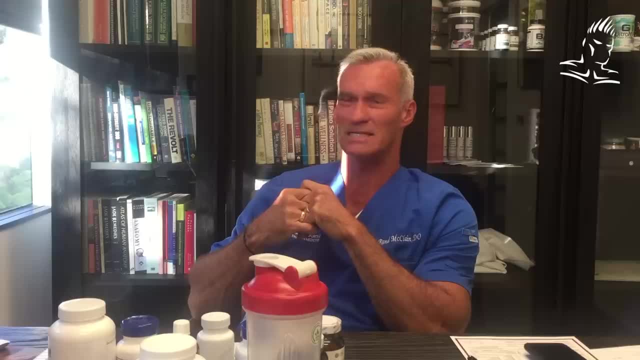 done properly, can be used very safely. it does has to have the potential, though, to convert to estrogen. so you know- i think we've talked about this before- not only if it were anavar, say, or a dht derivative like prima bull that didn't convert to estrogen. you're still displacing. 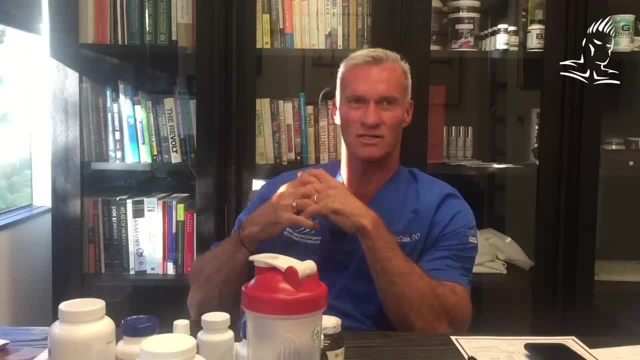 some of your naturally produced testosterone, or if you use some exogenous so that you still have to be concerned with conversion, but not conversion of the you know preemble in that case, or, or anavar, or whatever, but, um, again you've got the conversion from the actual steroid itself. 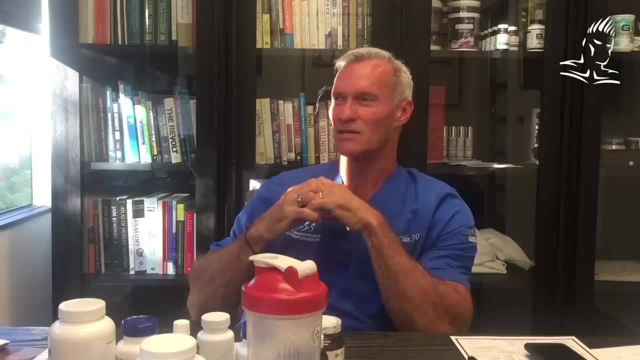 and also the conversion from the displaced testosterone is what i'm saying. yeah, so definitely would need to use some uh aromatase inhibitor as my preference or something to block the the estrogen. yeah, um, and that's it right. that's it. thanks for watching and i'll see you in the next talk.